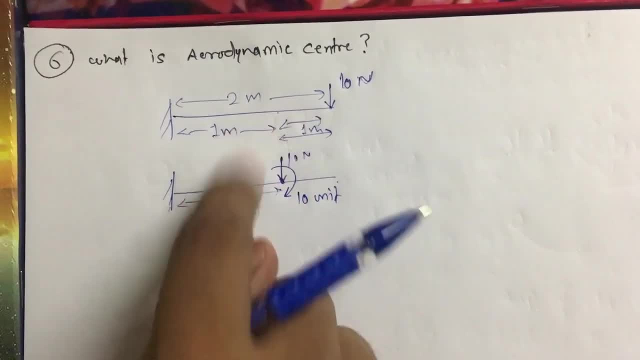 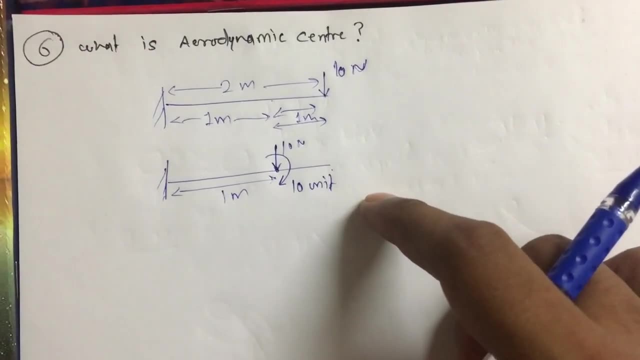 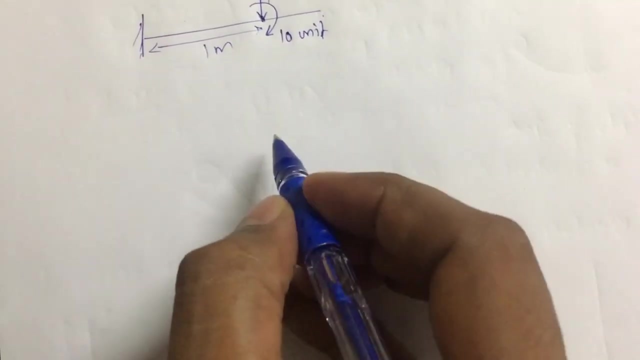 an extra moment whenever we shift our forces from one point to another point. So, with the help of same logic, I will explain what is called aerodynamic center. It is actually very, very easy, See, to understand aerodynamic center. suppose here you have, let us say, 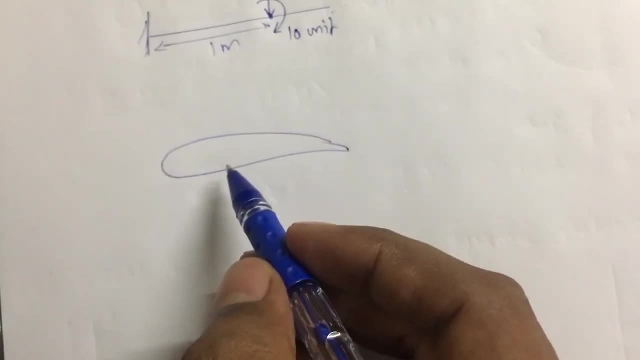 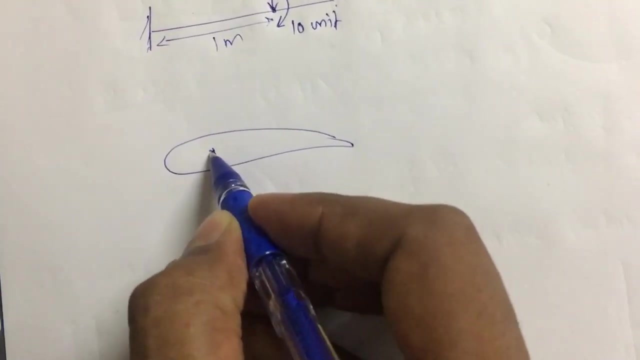 some airfoil. So two airfoils. I will talk at a time, but first. first, I will give you the logic. okay, Let me give the logic. fine, So suppose this is your CG and suppose this is your point. this point I am saying. 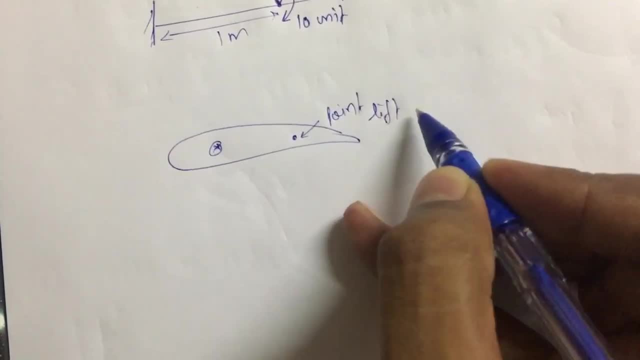 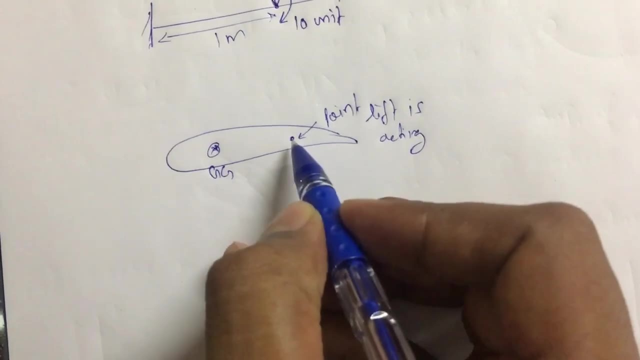 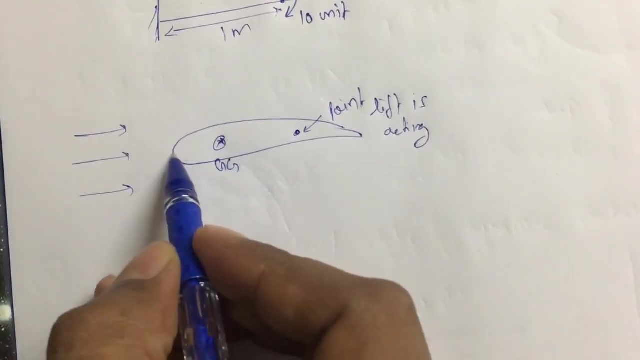 just a point: where lift is acting. where lift is acting Now, this is my CG. So, and the point here, some free stream is coming or actually, in reality, wing itself is moving, but I am considering this wing is in stationary state, So free streams are going like this. 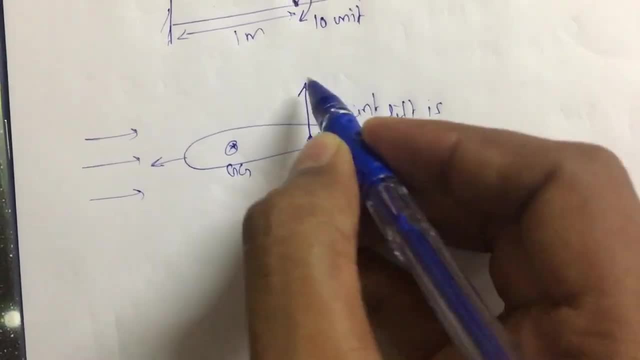 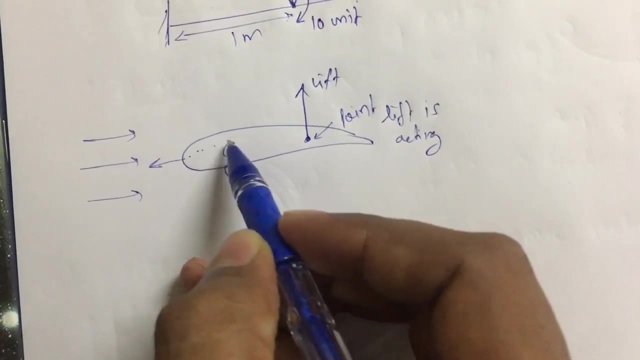 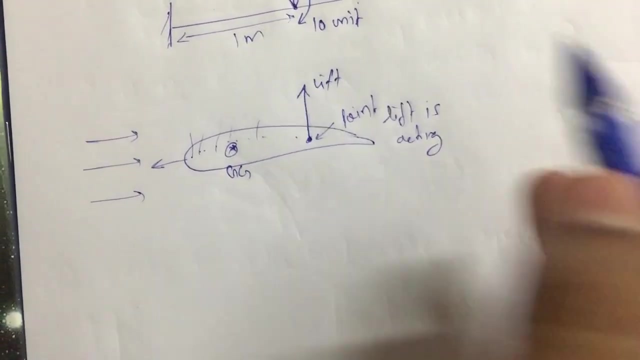 So at this point I will be having resultant lift. What is resultant lift? Because, see, every point will produce lift, right, So every point will produce lift. So, resultant of all the lifts I am showing, this is the lift. 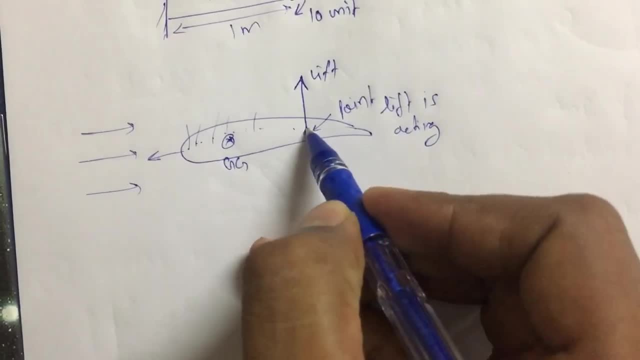 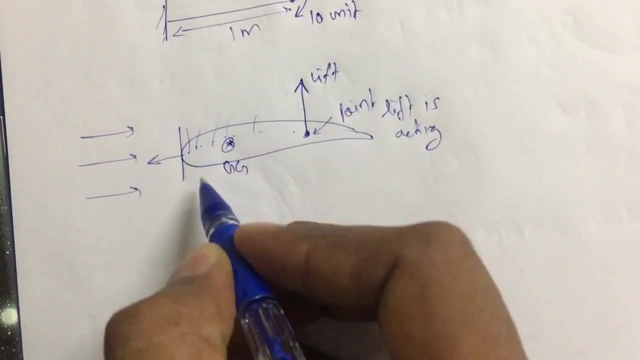 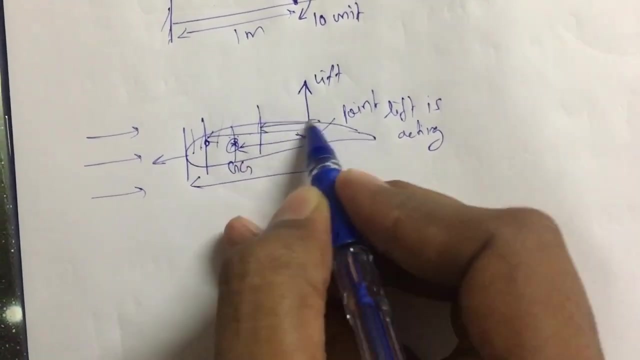 So this is the resultant lift. Now this lift will produce a moment about every point. I mean about this point also. I can find out the moment about this point also. I can find out the moment about CG also. I can find the moment about this point also, I can. I mean, 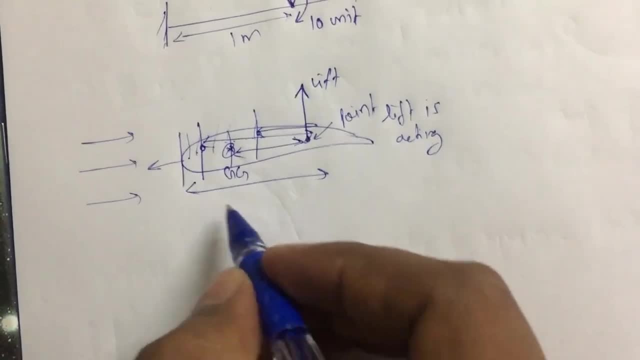 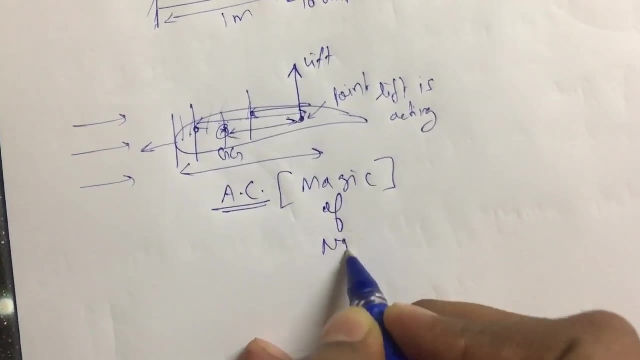 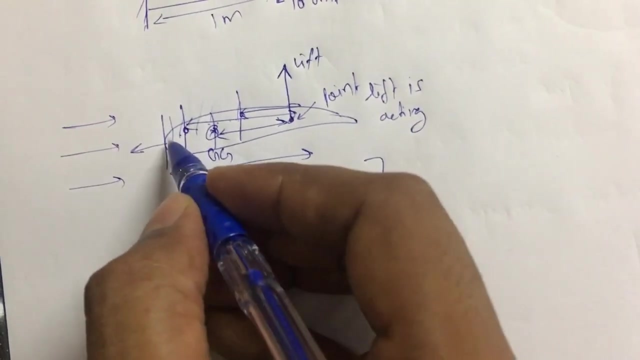 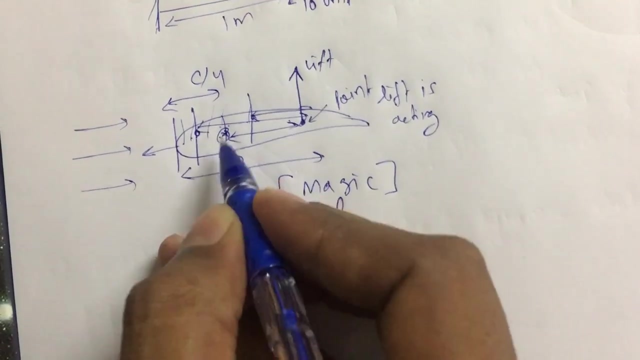 about all these points. I can find out moment Because we are talking about aerodynamic centre. so you must remember a word that is called magic, magic of the nature. Magic of nature means naturally. we have a point at c, by 4th location from the leading edge. I am not talking. 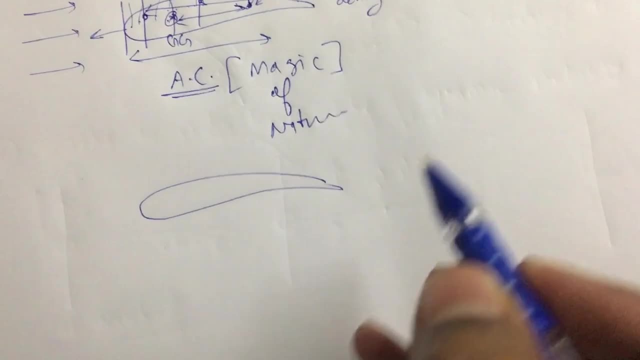 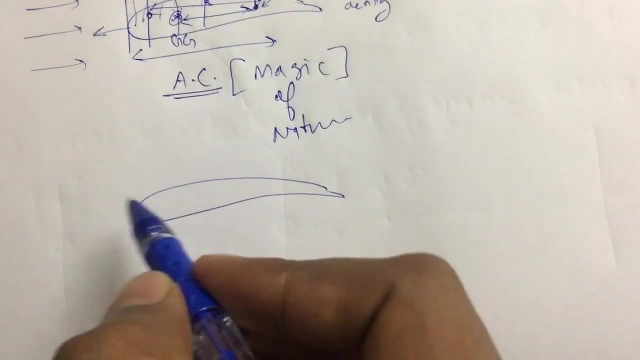 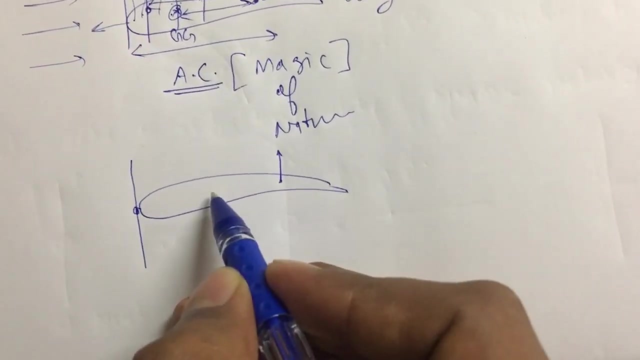 about CG. take a fresh diagram. This is airfoil and this is subsonic. airfoil c by 4 means subsonic. So this is the leading edge and this is your lift. Now I am not drawing CG here. CG was. 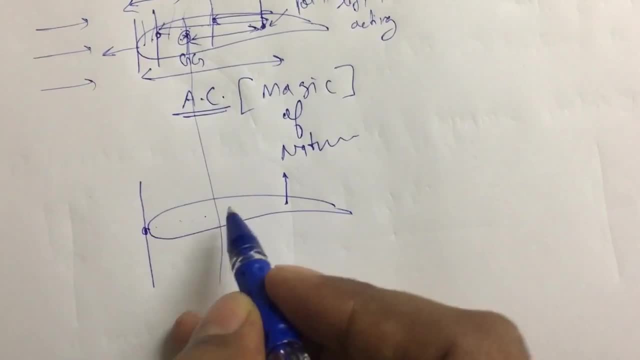 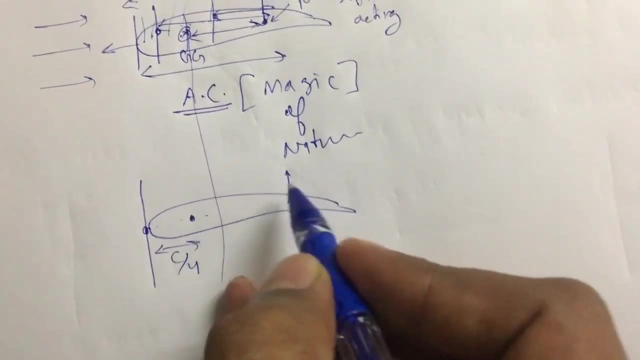 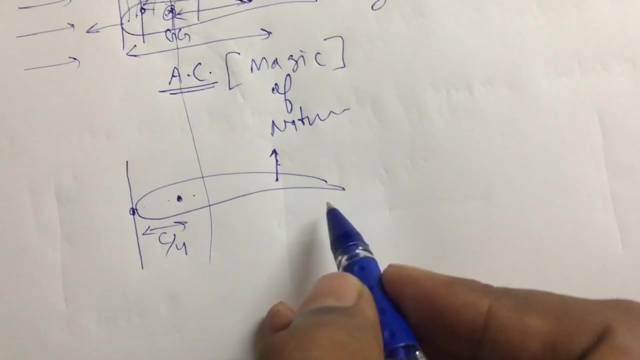 here somewhere. So I am saying we are having several points. So there will be a point at c by 4 about which you find out moment because of this lift. Now what to do? Change the angle of attack In the same case. change the angle of attack In the same case. change the angle of attack. 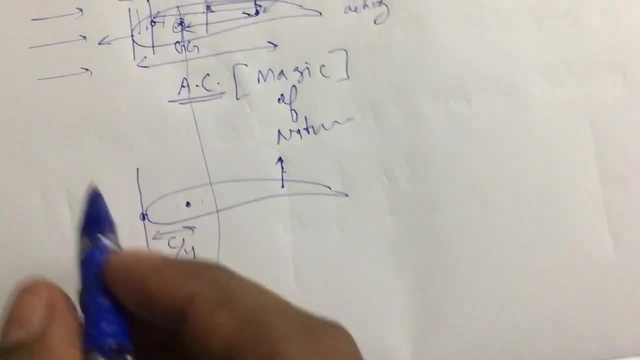 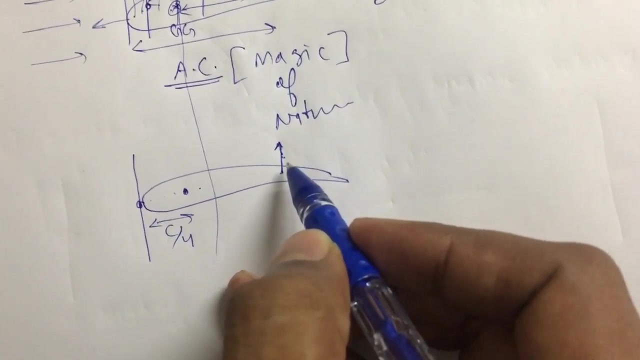 In the same case, change the angle of attack. Now, if you change the angle of attack, then what will happen? Location of this lift and amount of this lift, both will change, right? Location will also change and amount of the lift will also change. So suppose for the 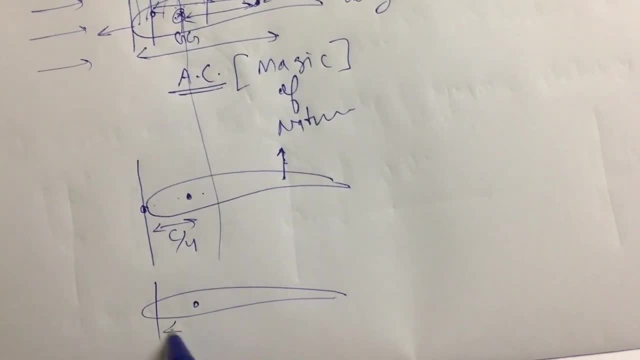 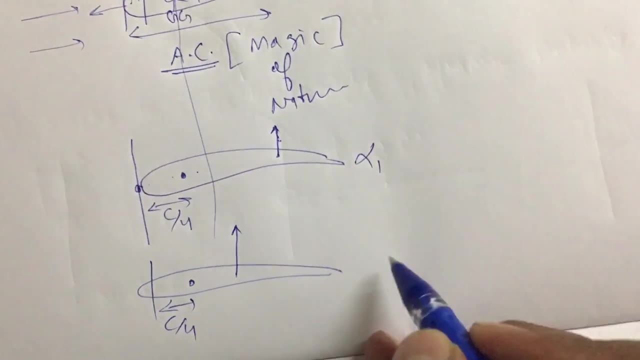 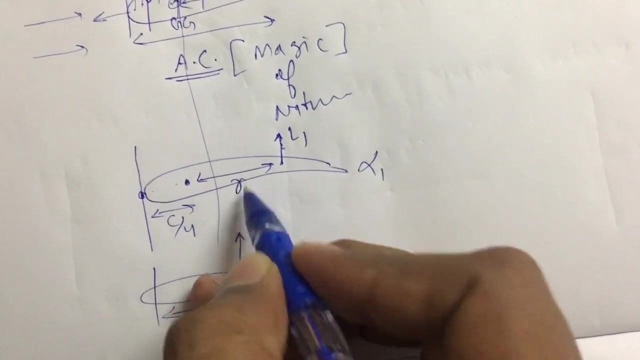 new case. still, this magical point is c by 4 and location of lift. suppose this is location of lift. So here angle of attack is alpha 1, here angle of attack is alpha 2.. So here. so here lift is L1, here lift is R2, here this distance is some R1, here this distance is some R2. 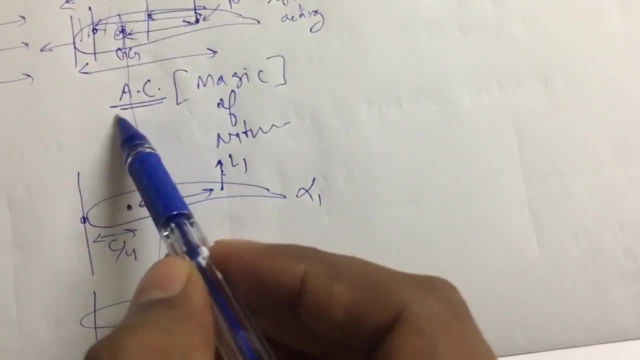 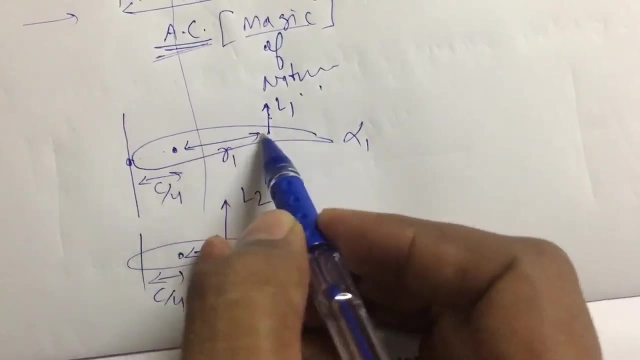 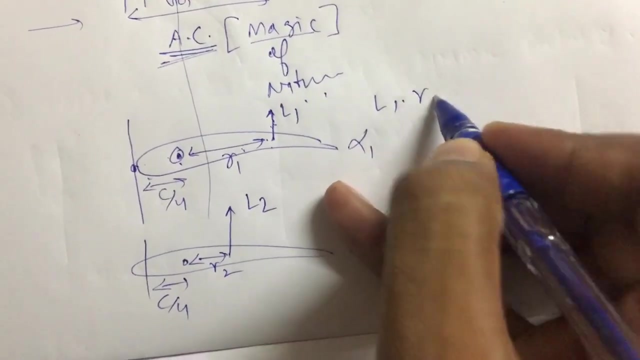 so why did I say aerodynamic center is magic of nature? because find out, lift in this case, sorry, find out moment about this point which is at c by 4, in this situation, which is nothing but L1 into R1. find out, in this case, which is nothing but. 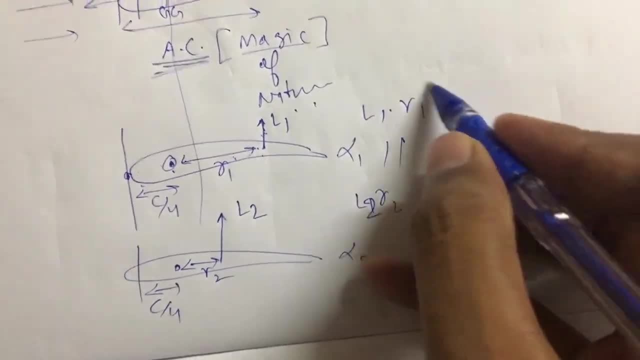 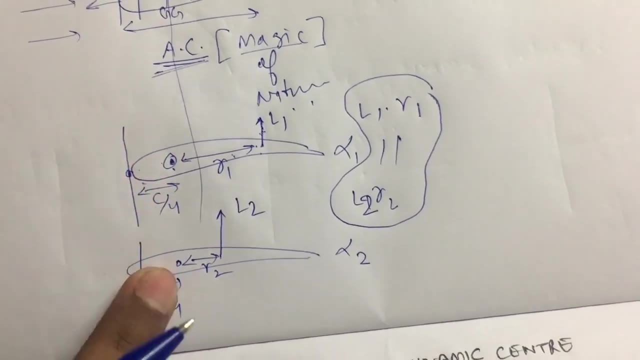 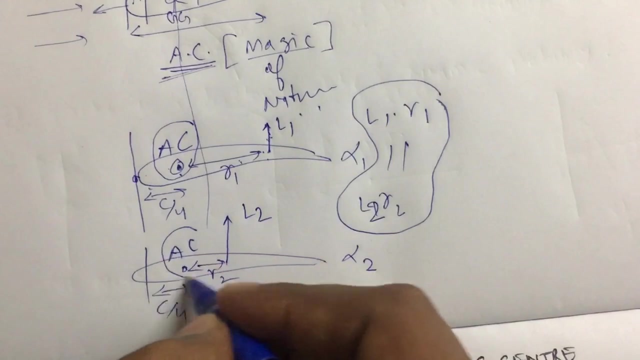 L1 into L2 into R2, right, so magically they both are same. so that's what we used to learn about: center of, sorry, aerodynamic center. so this point we say as aerodynamic center- this is word used by engineers in in this kind of cases like what is aerodynamic center? so that's why we 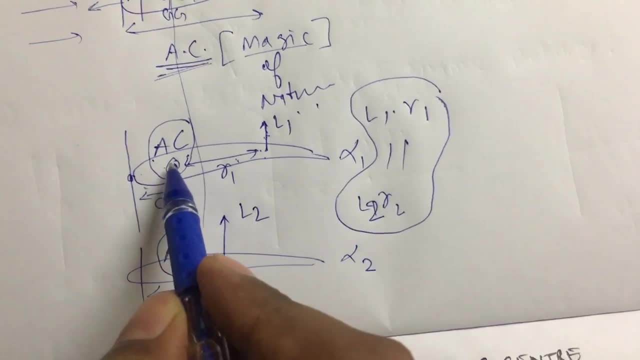 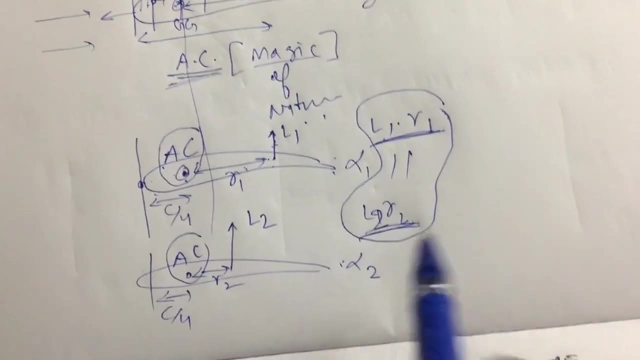 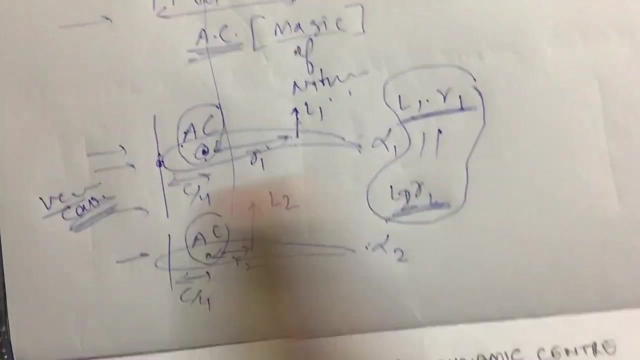 say, aerodynamic center is nothing but a point about which moment will be constant, even if you change the angle of attack. but but one thing you have to make sure in both the cases: velocity has to be constant. velocity has to be constant. make sure. so, when you are defining aerodynamic center, how will you say? 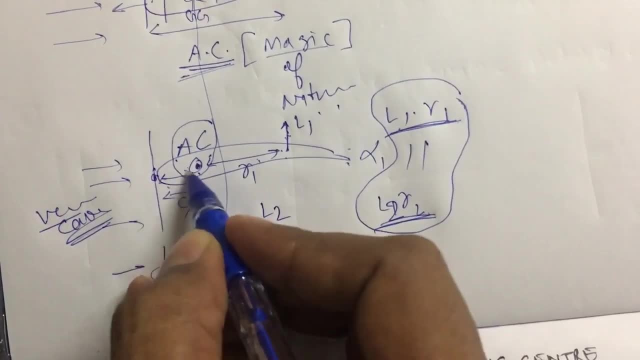 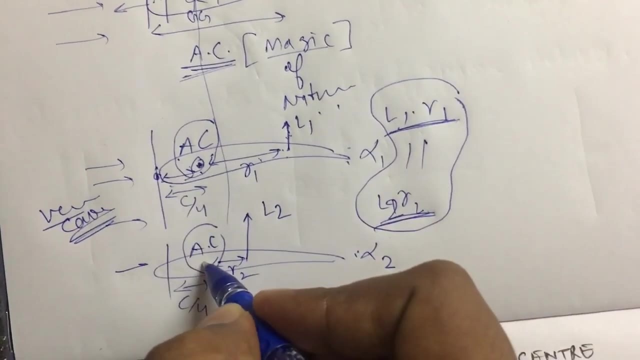 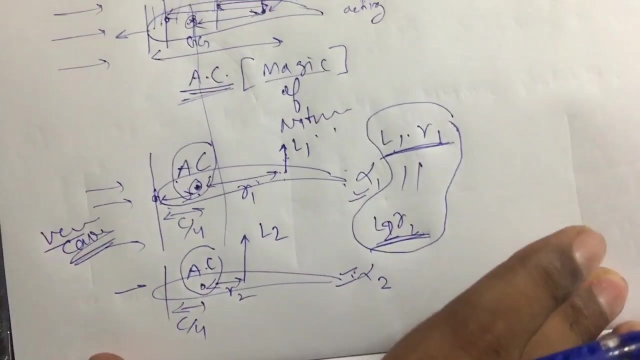 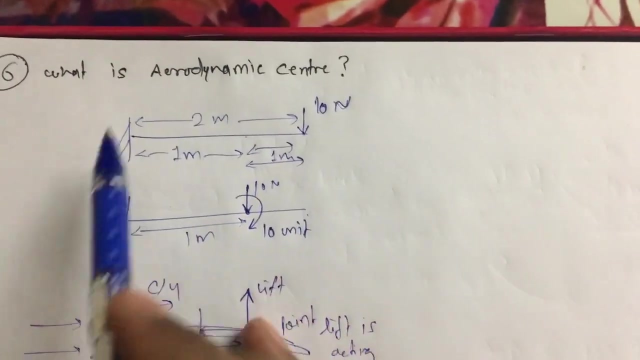 this is the aerodynamic center, is the point at quarter chord from the leading edge about which moment is constant with respect to angle of attack. I hope you got it and basic idea already you are having because of your university courses. now one additional thing I will use here like I give: I give this thing right. so 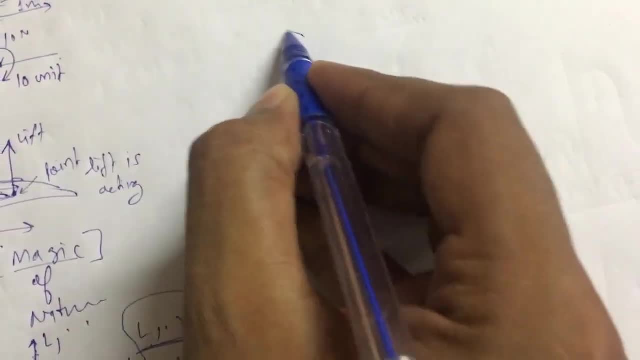 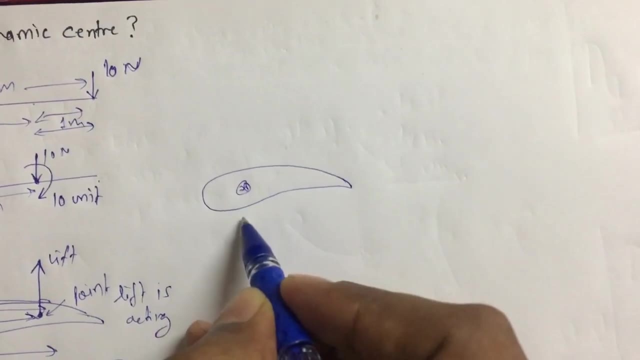 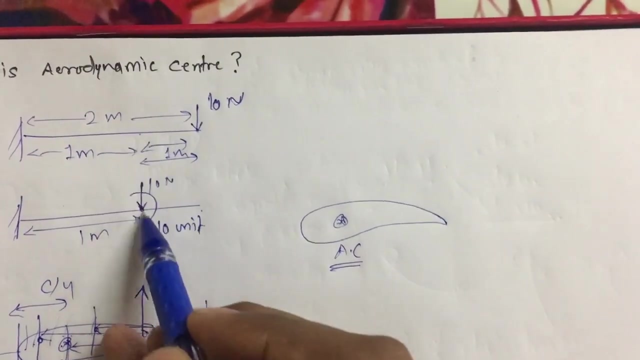 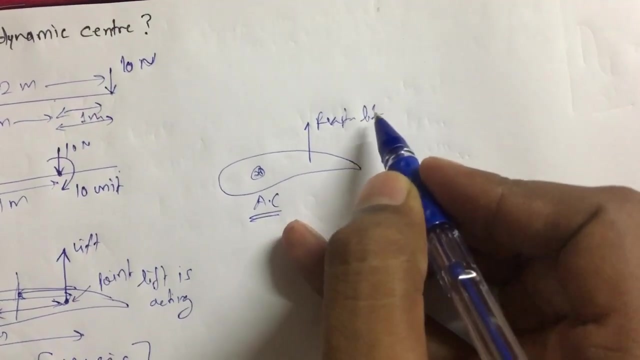 same thing I will produce here also. so if you are having a airfoil and in this airfoil you have your aerodynamic center, okay, so, like in this case, I shifted my force from here to here. same I had some predator meals usually need to lift or density lifted. 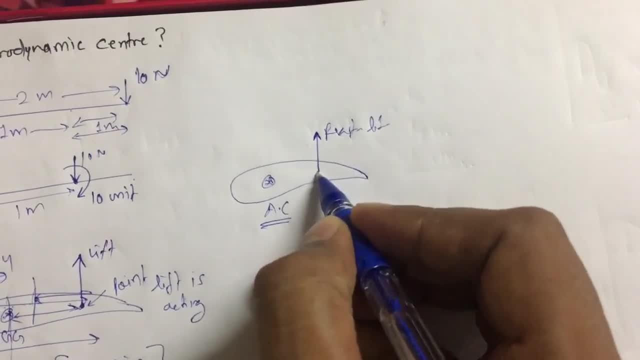 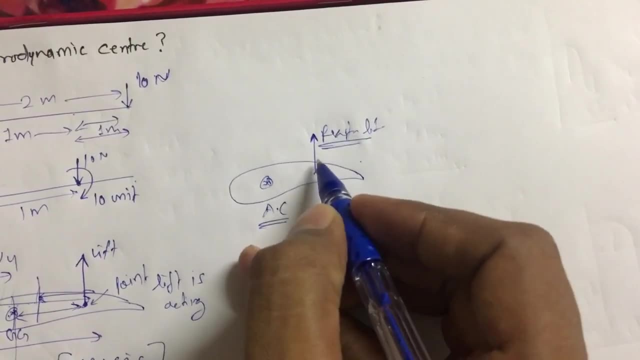 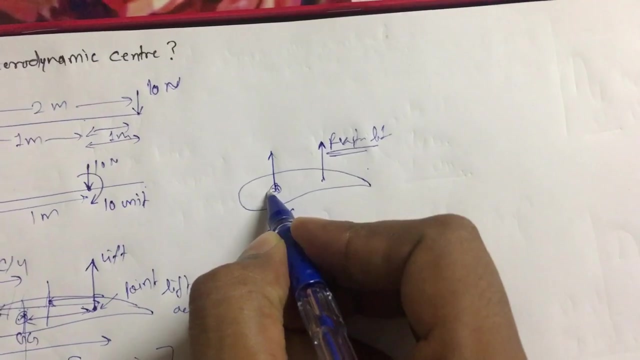 is nothing but the point of center of pressure. okay, at center of pressure, only ready to lift, we'll work, and it will work well, seeing this different dynamic force and put your and put your. so if we have shifted, then what would you have to shoot? you have to. 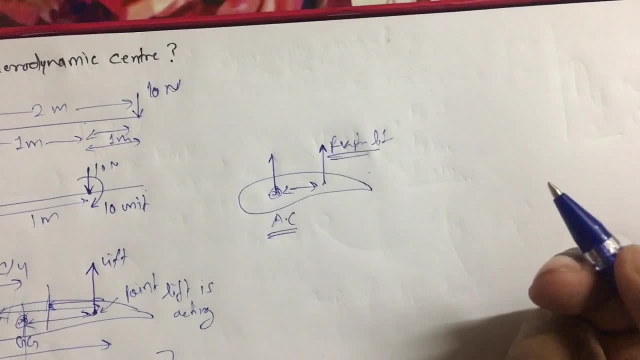 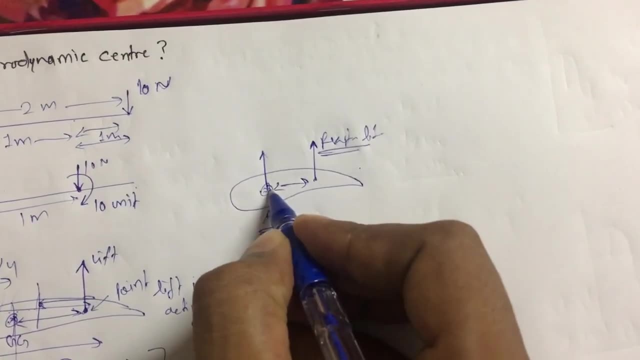 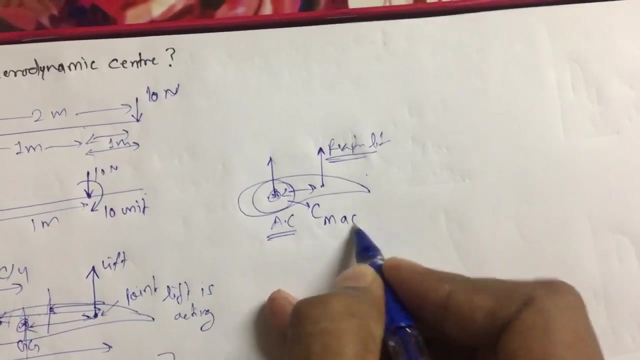 shift this much momentum also. so that moment, wife, that's why I just said shift also. you shift, that's all done and you got it. now, what is your dynamic center? so, because you are shifting the moment here, you are shifting the moment here. so this moment will be just just to show the moment as CMAC. CMAC means: 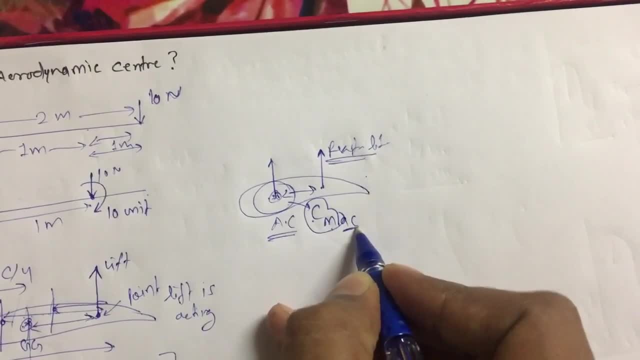 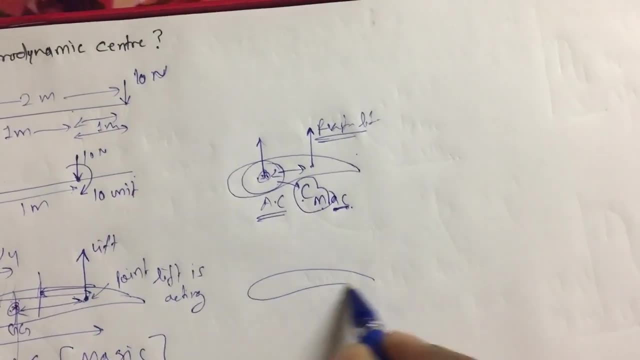 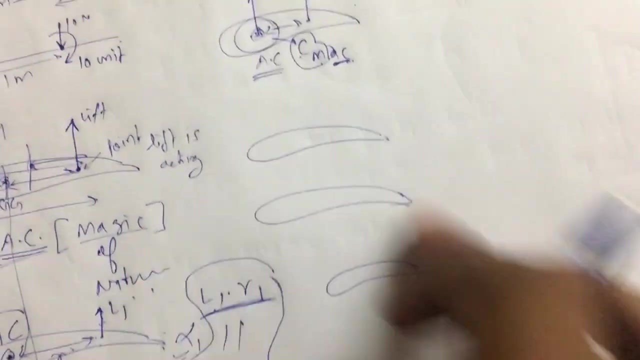 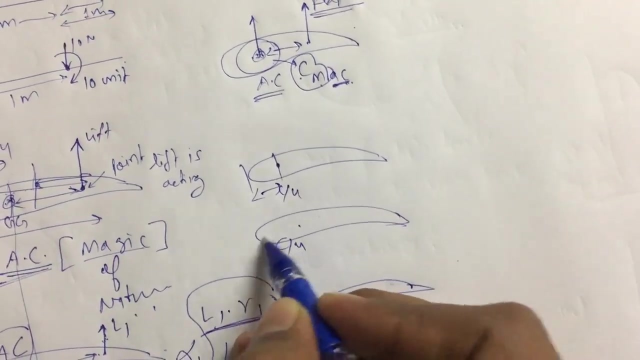 coefficient of moment at a dynamic center, got it. so now suppose you are having several airfoils, different airfoils. I mean same airfoil, similar, say exactly same diagrams are different, different. so suppose you are having that magical point C by 4, C by 4, C by 4, again this point C by 4, so, but they are at. 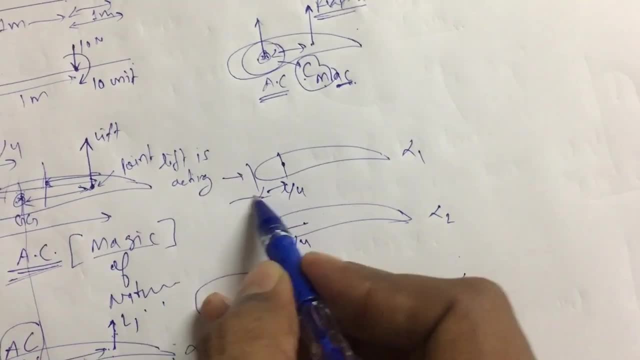 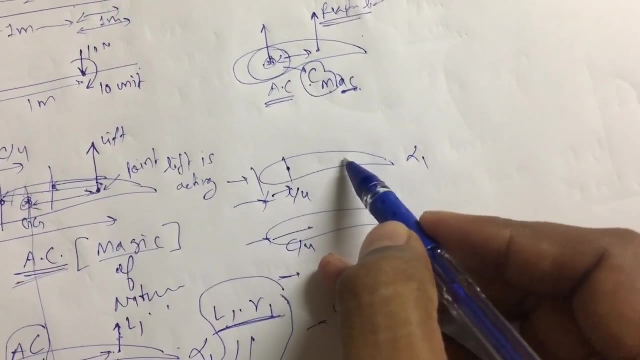 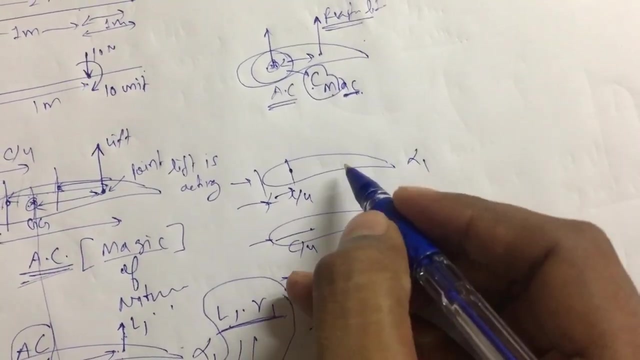 different, different angle of attacks. and what is constant here? the flow velocity, uniform free stream velocity. that is constant. so in this case center of pressure will be somewhere else. okay, let me explain what is center of pressure. center of pressure is nothing but the point where is retent lift is working, actually not resultant lift, resultant aerodynamic. 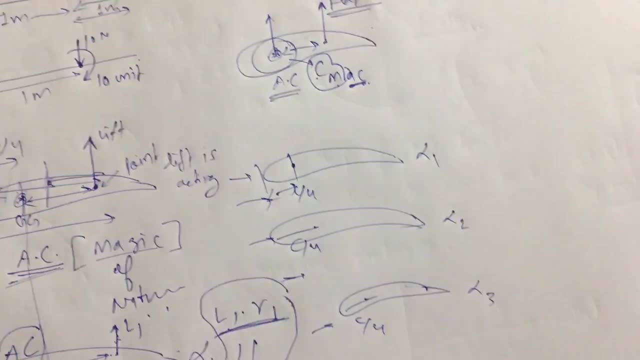 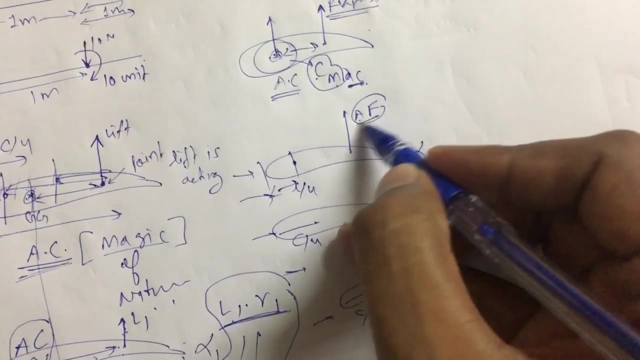 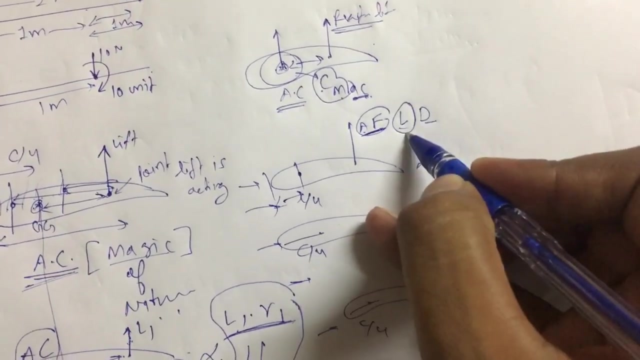 force is working. that point is called center of pressure. so suppose at this point aerodynamic force, aerodynamic force, make sure, is working. aerodynamic force is having two component, one is lift and one is drag. okay, so sometimes we only refer lift, lift, lift, lift. so we say lift, lift, lift. so aerodynamic force is having